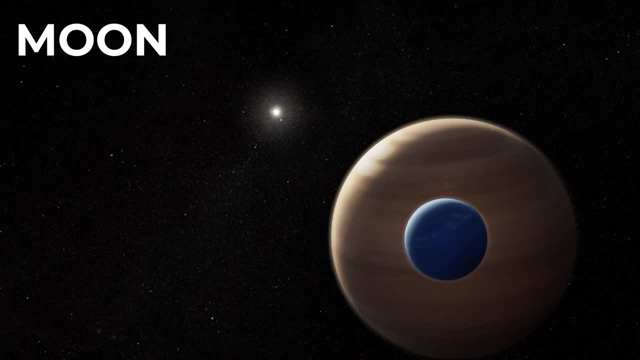 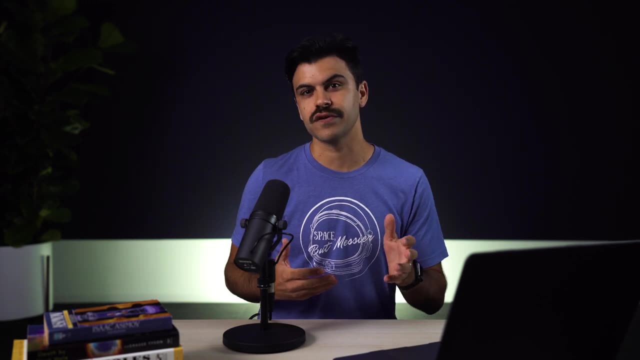 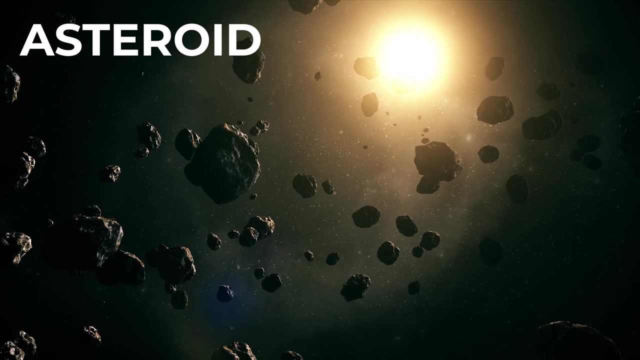 fight me is designated. a dwarf planet, A moon or a satellite is an object that orbits a planet. The term satellite is also used more generally to refer to any object orbiting another object. An asteroid is a relatively small and rocky object that orbits a star. 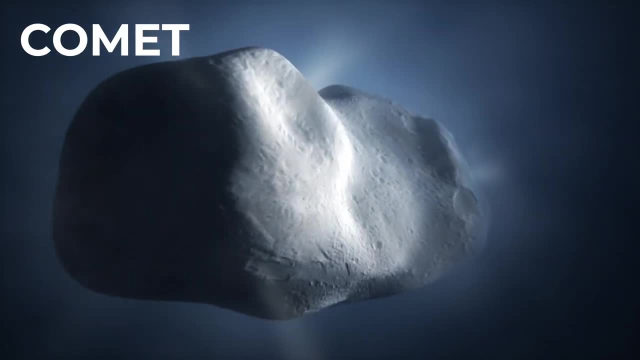 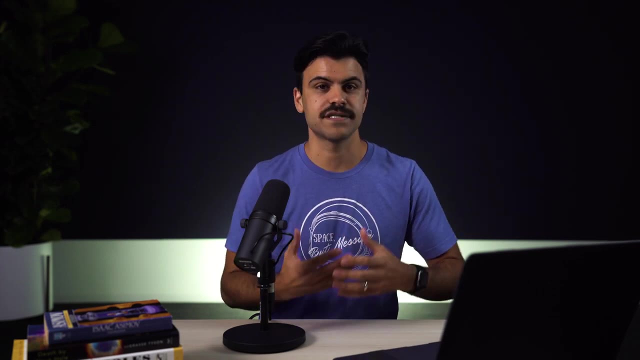 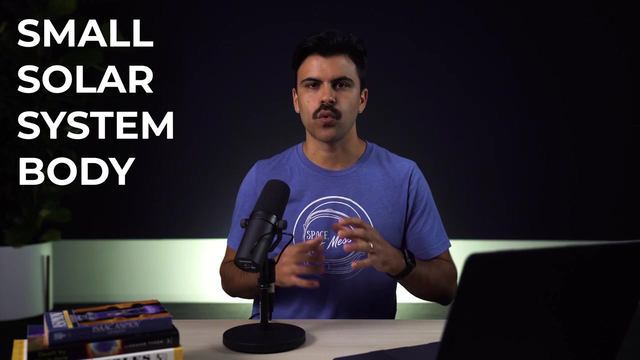 Whereas a comet is a relatively small and ice-rich object that orbits a star. So asteroids and comets are very similar. Asteroids are rocky, comets are icy, but they both orbit a star. A small solar system body is an asteroid, comet or other object that orbits a star. 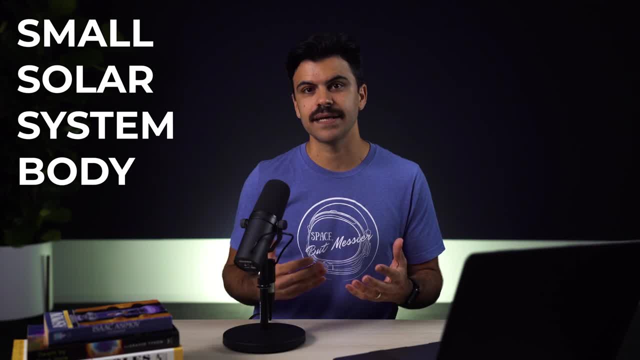 but is too small to qualify as a planet or a dwarf planet like Pluto. Next, let's touch on some collections of astronomical objects. The solar system is the Sun, the Moon and the Earth. The Sun is the sun, the Moon is the moon and the Earth is the moon. 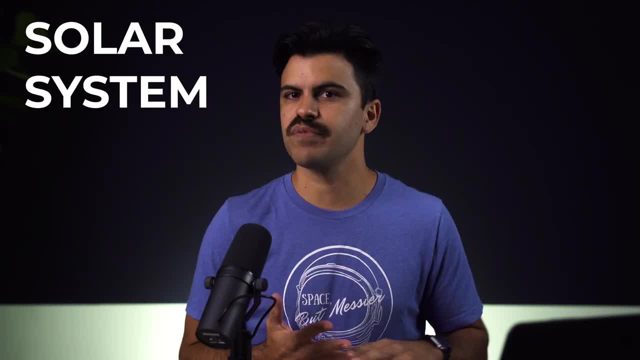 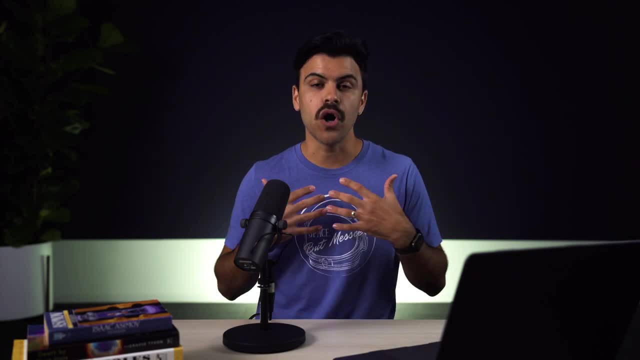 The Sun is the sun, the Moon is the moon and the Earth is the moon. The Sun is the moon and the Earth is the moon And all the material that orbits it, including planets, dwarf planets and small solar system bodies like asteroids and comets, Although the term solar system technically refers only to our. 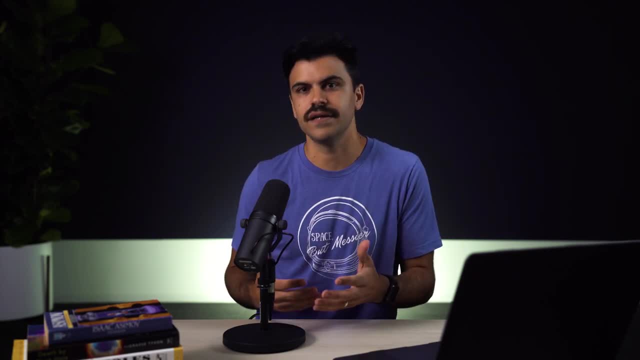 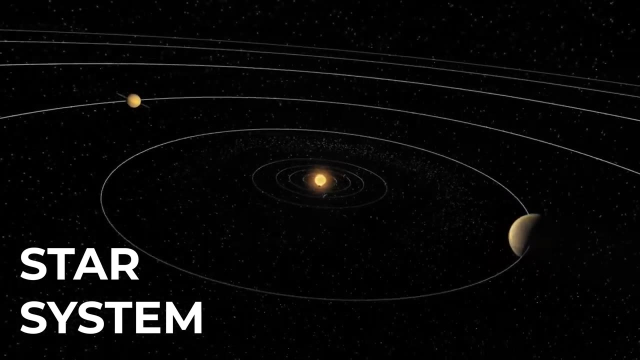 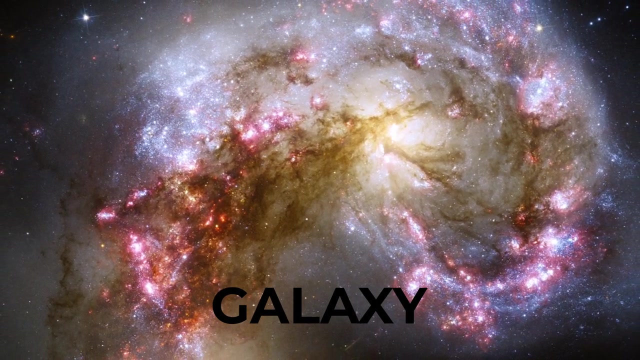 own star system because solar means of the sun. it often applies to other star systems as well. A star system is a star, sometimes more than one star, and any planets or other materials that orbit it. A galaxy is a great island of stars in space, all held together by gravity and orbiting. 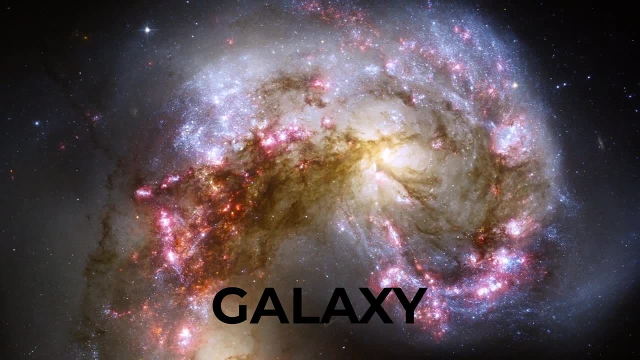 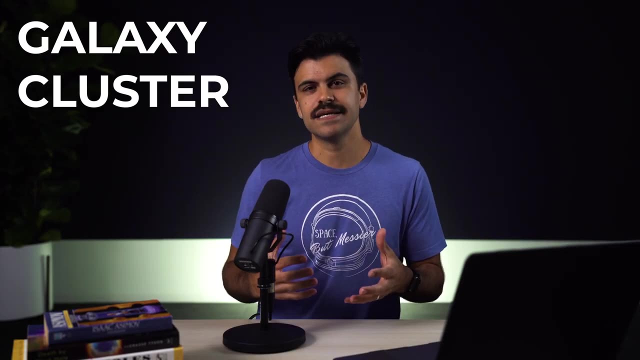 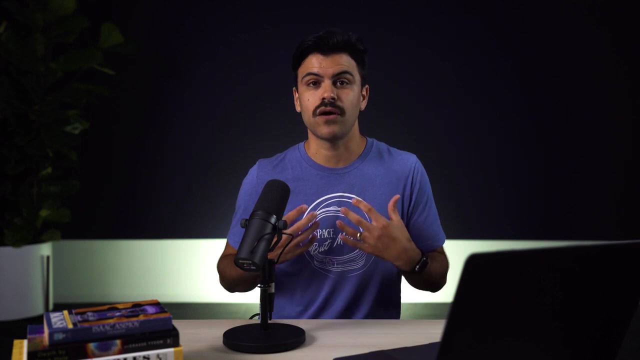 a common center with a total mass equivalent to millions, billions or even trillions of stars. A cluster of galaxies or a group of galaxies is a collection of galaxies bound together by gravity. Small collections, up to a few dozen galaxies, are generally called groups, like our local group. 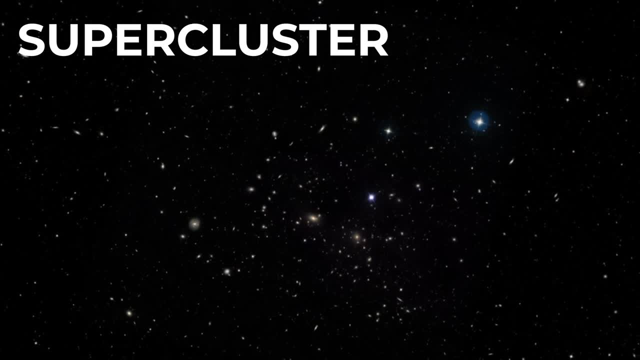 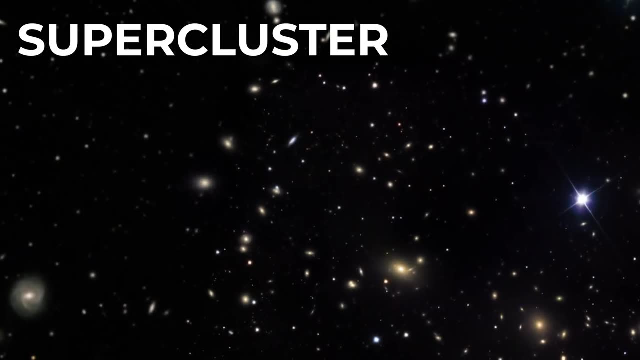 while larger collections are called clusters. A supercluster is a gigantic region of space in which many groups and clusters of galaxies are packed more closely together than elsewhere in the universe. A supercluster is a gigantic region of space in which many groups and clusters of 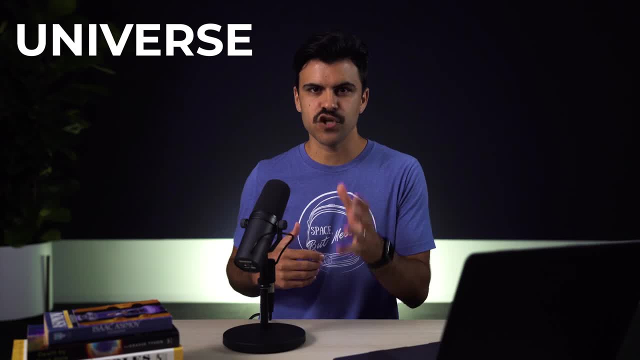 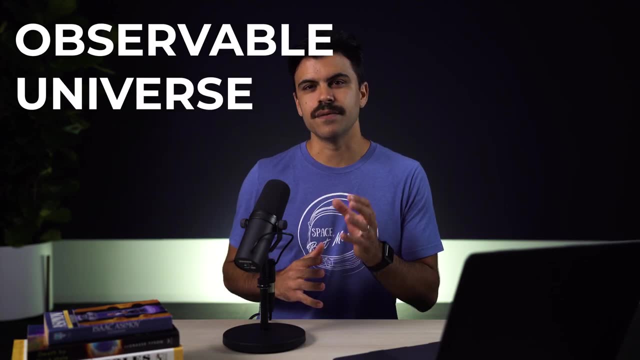 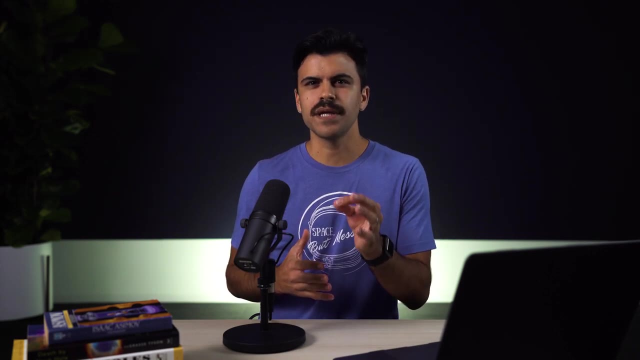 galaxies are packed more closely together than elsewhere in the universe. The universe is the sum total of all matter and energy, that is, all galaxies and everything between them. The observable universe is the portion of the entire universe that can be seen from Earth, at least in principle. The observable universe is probably only a tiny portion of the.